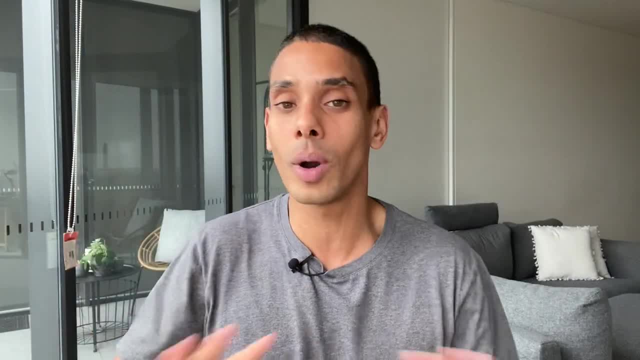 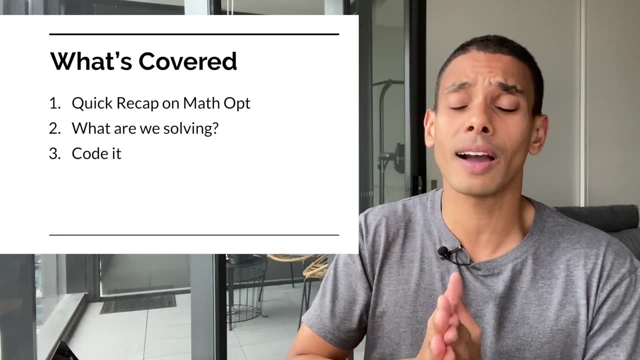 and constraint-based programming. Now you're probably thinking: what the hell is that? Well, don't fret, We're going to go through all of that in a second. So let's get to it Now. we're going to be covering a bunch today, but specifically we're going to be covering 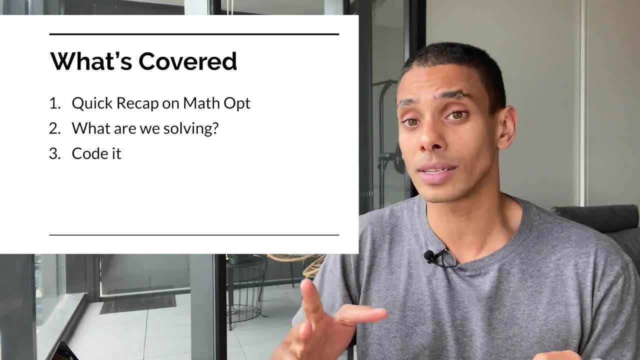 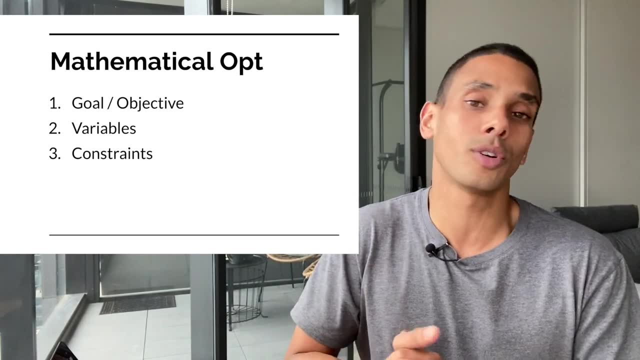 what mathematical optimization is the problem that we're trying to solve and, last but not least, we're actually going to code it up. So what is mathematical optimization? There's three key things that you need for any good mathematical optimization problem. These are a goal or an. 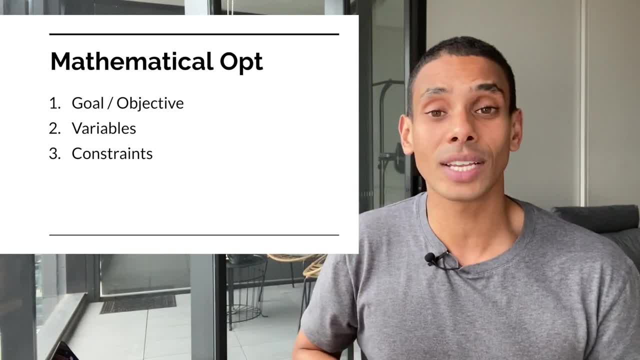 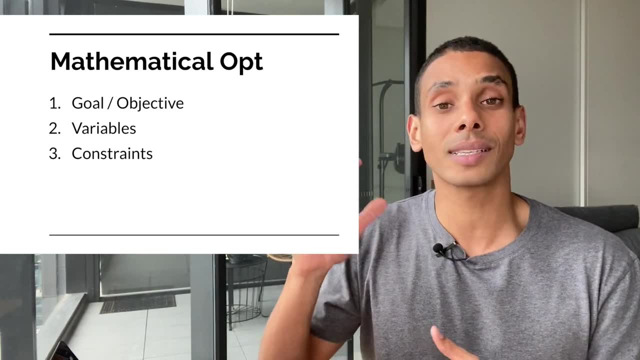 objective: your variables or levers that you can change and, last but not least, your constraints. So you're trying to find an optimal value for your variables or your levers so that you can maximize or minimize your goal and stay within your specific constraints. A good example of this: 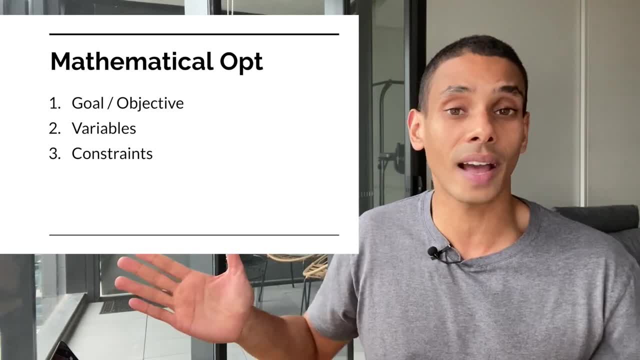 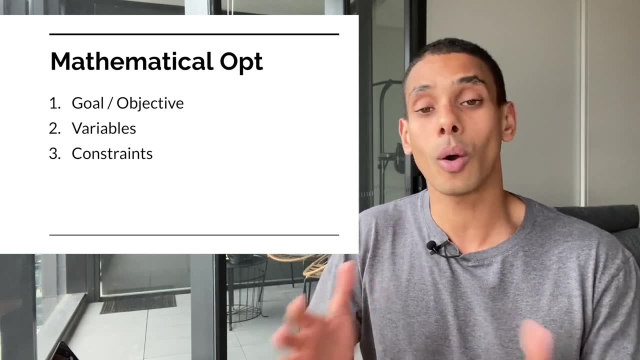 is: how much of each product should we produce if we've got a constrained factory floor? Now another really good example is: how should we schedule people on a roster so that we maximize our productivity but we also meet the requirements of our scheduling process? 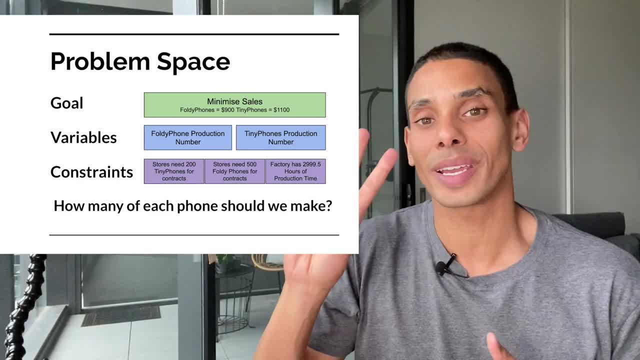 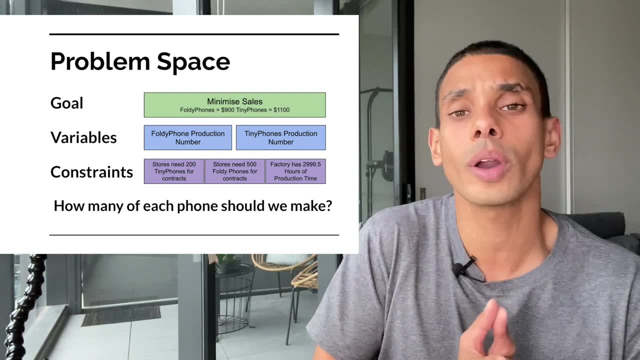 Now, the specific problem that we're going to be solving again has three key things. It has goals, variables and constraints. Now, in our particular case, we're helping at a phone factory and we're trying to work out how many phones of each model that they have should we generate in order to 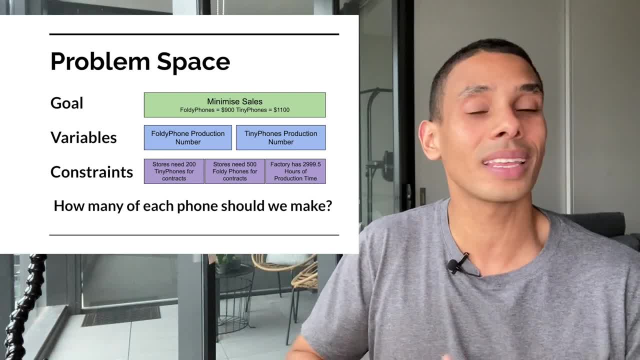 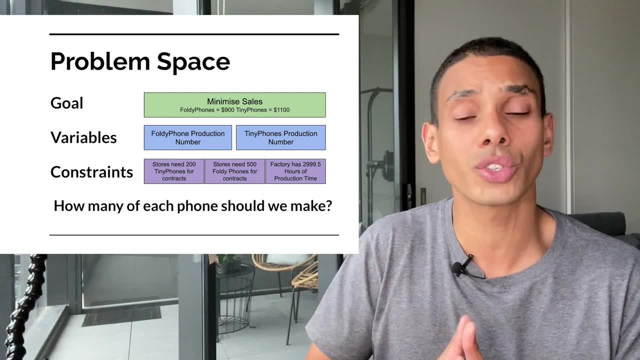 maximize our sales. Now, in our particular problem, we're assuming that they sell all of the phones that they have. Ideally, we want to make the phones that are ideally the most profitable. Now our core constraints are that we have a minimum level of production that we need to meet in order to hit 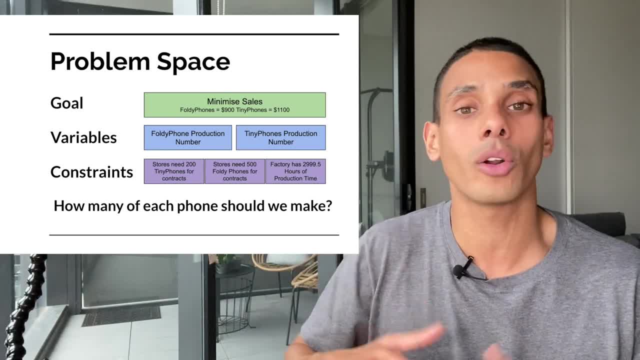 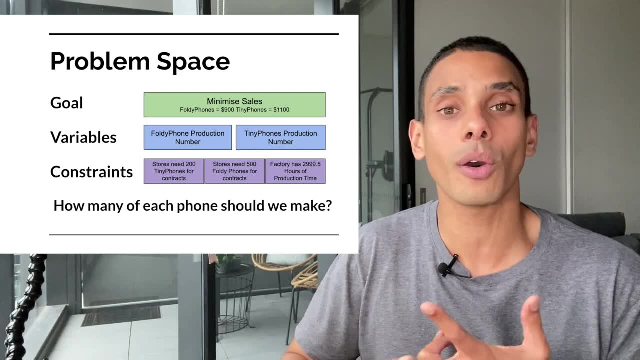 our contractual requirements, but we also have a cap on how many hours that we have to generate products within our factory. So in this case, we need to work out how many tiny phones and how many foldy phones we should make in order to maximize our overall sales. Enough theory, let's get into. 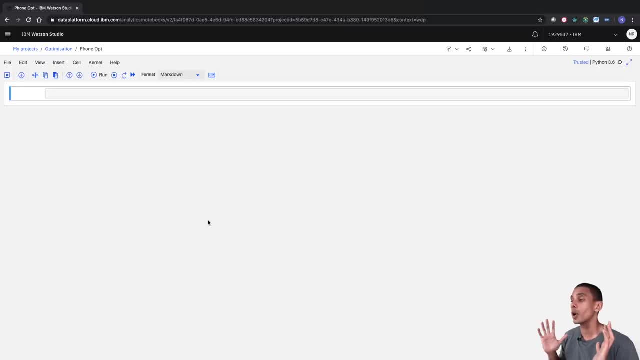 the code. So let's get started solving our problem Now. we're going to be working in a Jupyter notebook for this, So first up, what we're going to do is lay out our problem Now, remember, a mathematical optimization problem has three key things. Those are goals, variables. 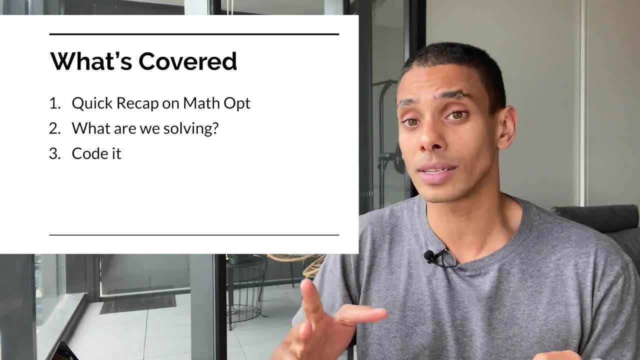 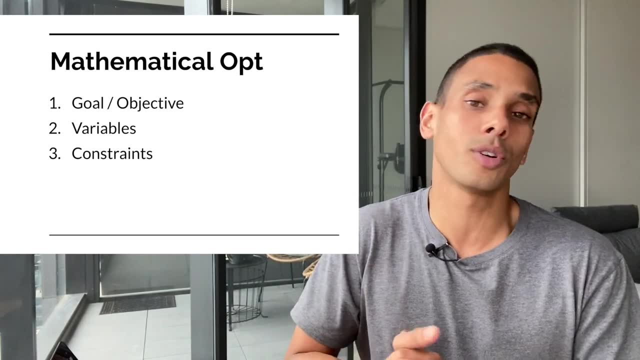 what mathematical optimization is the problem that we're trying to solve and, last but not least, we're actually going to code it up. So what is mathematical optimization? There's three key things that you need for any good mathematical optimization problem. These are a goal or an. 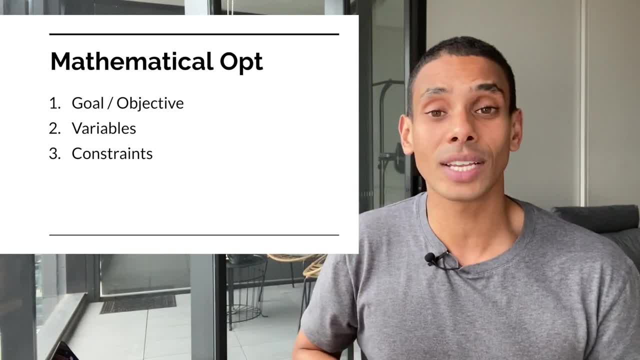 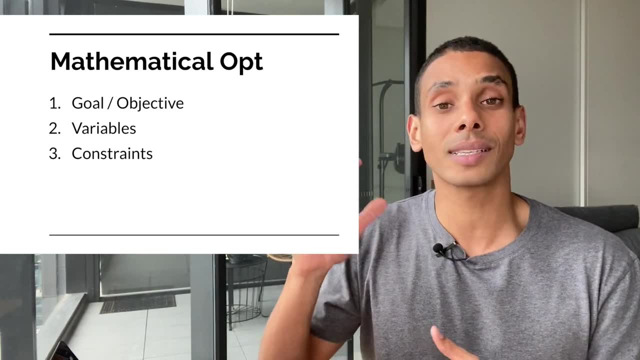 objective: your variables or levers that you can change and, last but not least, your constraints. So you're trying to find an optimal value for your variables or your levers so that you can maximize or minimize your goal and stay within your specific constraints. A good example of this: 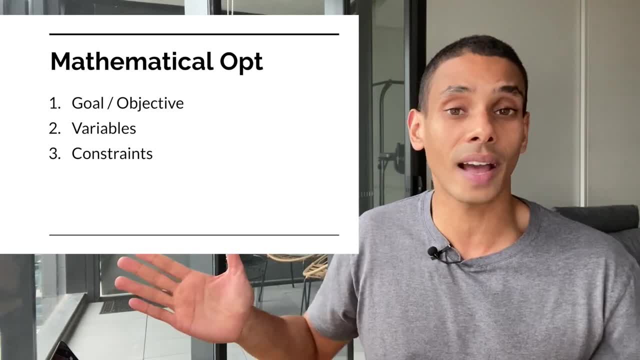 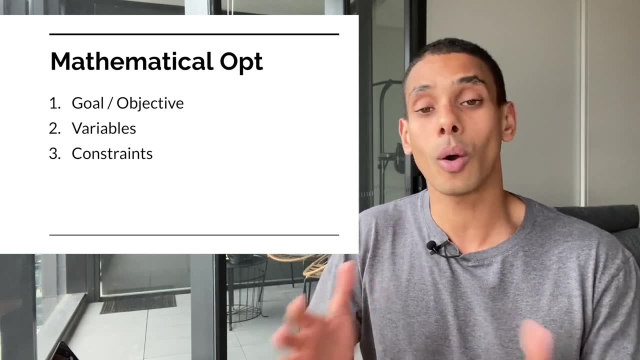 is: how much of each product should we produce if we've got a constrained factory floor? Now another really good example is: how should we schedule people on a roster so that we maximize our productivity but we also meet the requirements of our scheduling process? 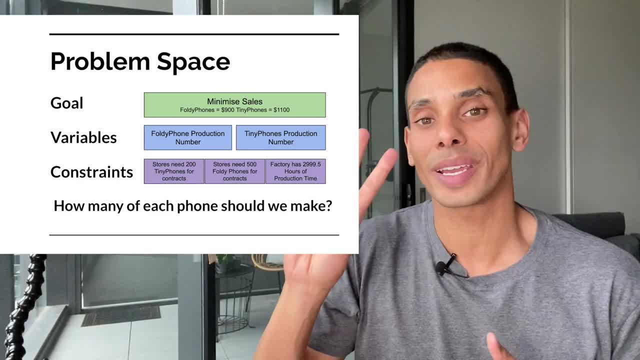 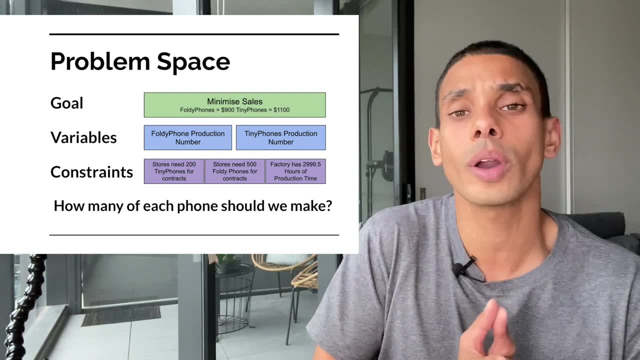 Now, the specific problem that we're going to be solving again has three key things. It has goals, variables and constraints. Now, in our particular case, we're helping at a phone factory and we're trying to work out how many phones of each model that they have should we generate in order to 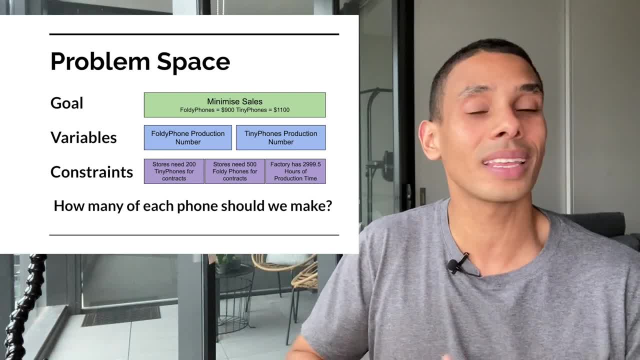 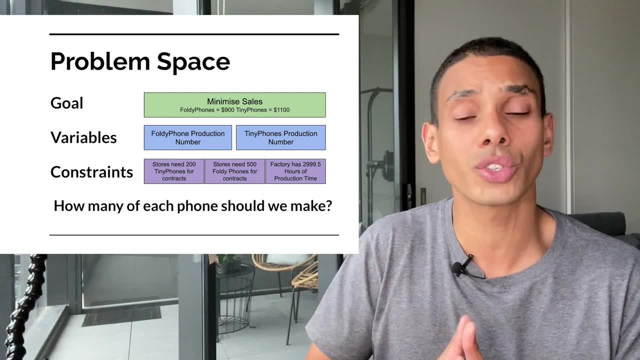 maximize our sales. Now, in our particular problem, we're assuming that they sell all of the phones that they have. Ideally, we want to make the phones that are ideally the most profitable. Now our core constraints are that we have a minimum level of production that we need to meet in order to hit 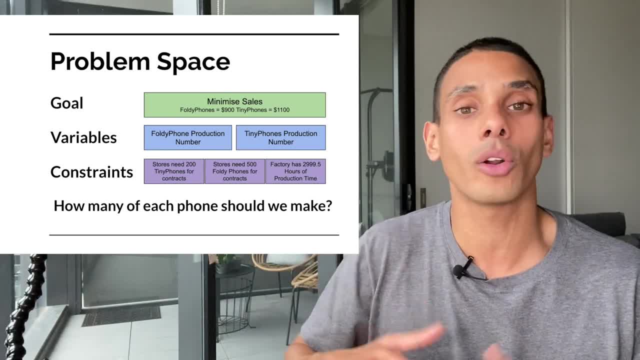 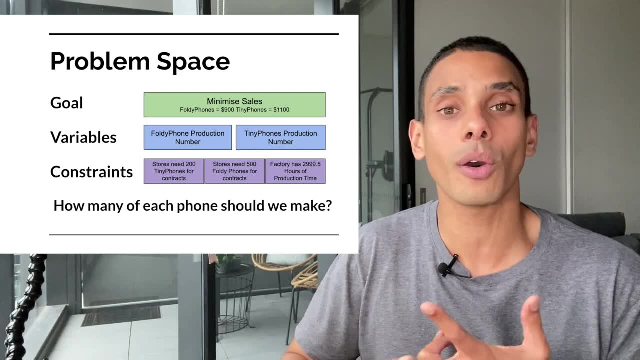 our contractual requirements, but we also have a cap on how many hours that we have to generate products within our factory. So in this case, we need to work out how many tiny phones and how many foldy phones we should make in order to maximize our overall sales. Enough theory, let's get into. 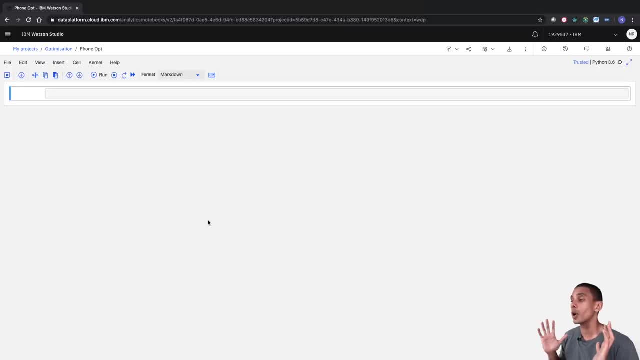 the code. So let's get started solving our problem Now. we're going to be working in a Jupyter notebook for this, So first up, what we're going to do is lay out our problem Now, remember, a mathematical optimization problem has three key things. Those are goals, variables. 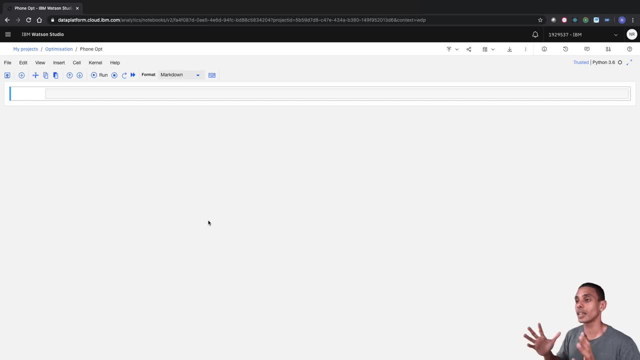 and constraints. So what we're going to do is just lay out our notebook to give it a little bit of a framework to surround that. So let's go ahead and add in some new cells. So in this case, we're going to add in first up, we're going to add in a cell for our variables. 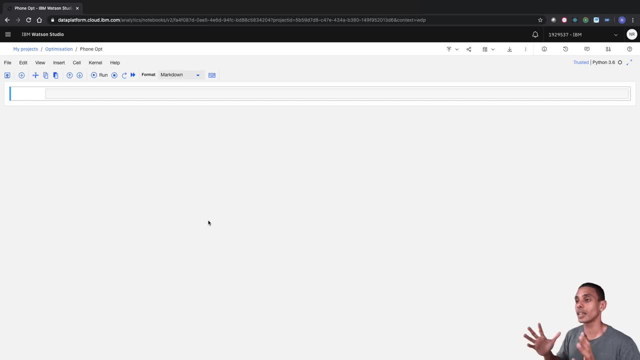 and constraints. So what we're going to do is just lay out our notebook to give it a little bit of a framework to surround that. So let's go ahead and add in some new cells. So in this case, we're going to add in first up, we're going to add in a cell for our variables. 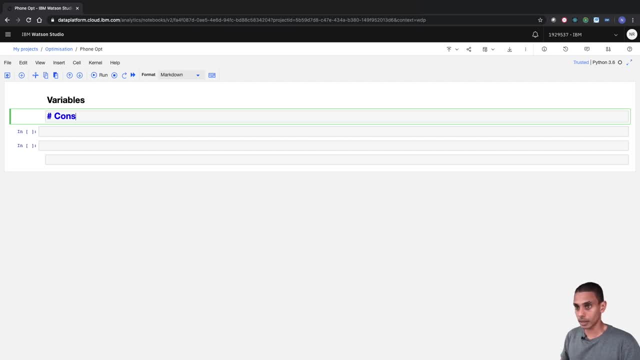 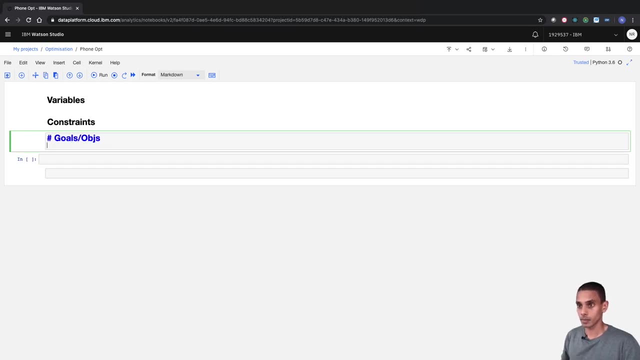 and then we're also going to add in a markdown cell for our constraints, but, not least, we're going to add one for our goals or objectives. Perfect Now, in terms of our variables. we've got a couple of key ones. So, before we actually go and build those variables, 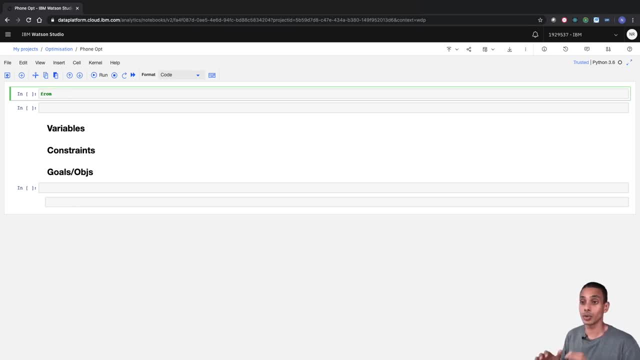 what we want to do is import our dependencies. So to do that we're just going to use the docplex package. So this sort of has a really powerful solver behind it, So that's going to allow us to solve a mathematical problem. So let's import docplex and then from mp and model 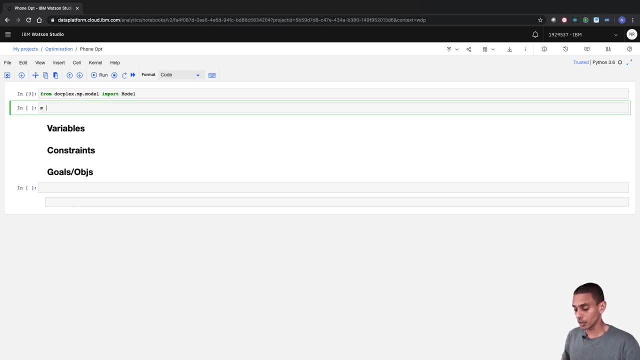 we're going to import the model class. What we're going to do is create an instance of the model, So everything is going to be attached to our model and think of your model as your problem, really. So we'll create a model. 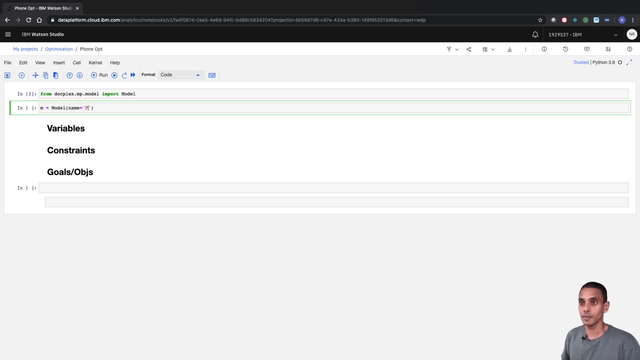 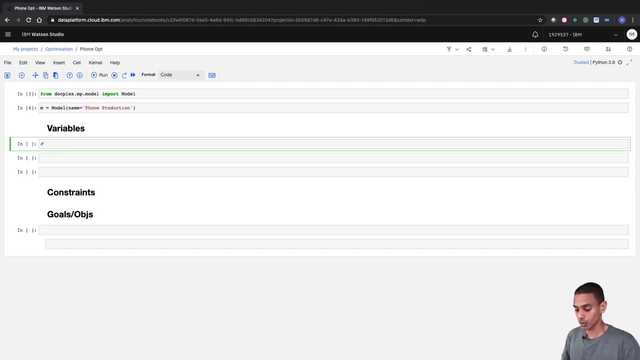 and we're going to name it phone production. and then, within our variables, we're going to name a couple of variables. So, first up, what we're going to do is we're going to create our phone production variables, right? So we have two classes of phones. We had our foldy phone. 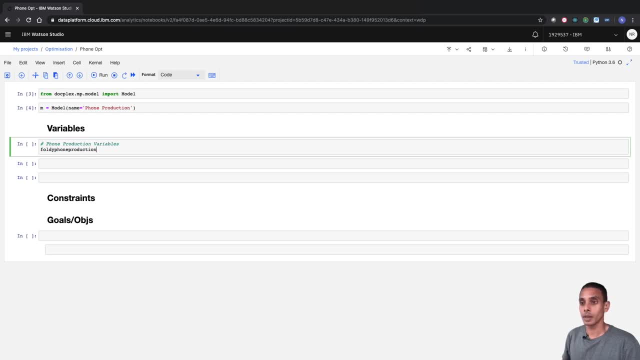 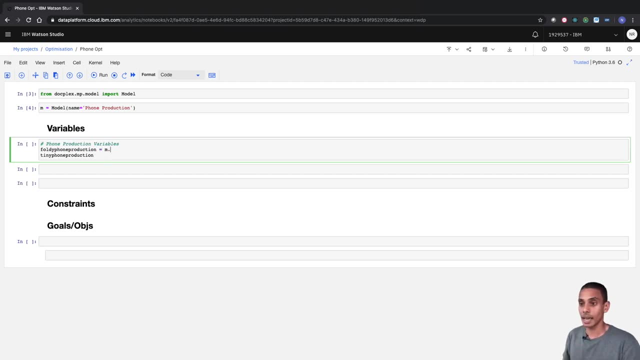 and we had our tiny phone. So let's create two variables for that and add our tiny phone production. Now to create a variable with docplex, all we need to do is type in mcontinuousvariable and we're going to name this as well. So we'll name it foldy. 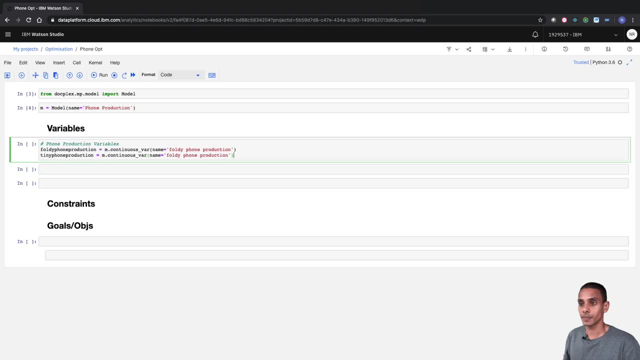 And what we can do is copy that to our tiny phone and rename that tiny phone production- Cool. So we've got our two production variables. Now we had a couple of constants as well that we didn't mention in our problem formulation statement. So what we're going to do is we're 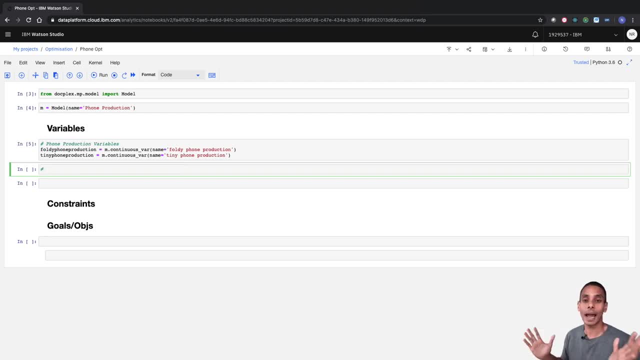 going to do, or our key constraint is really how much time we've got within our manufacturing plant to actually create these phones. So what we want to do is set up a variable that contains how long it actually takes to generate or create one of these phones. So let's create two variables for 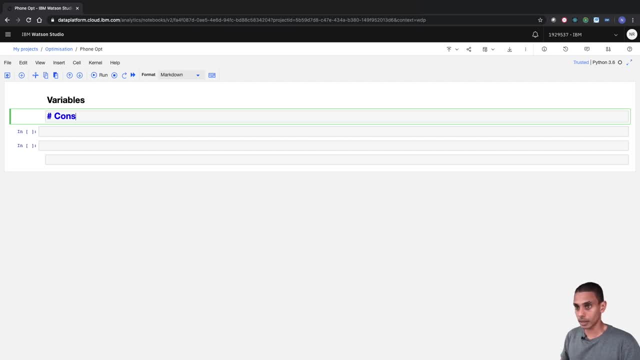 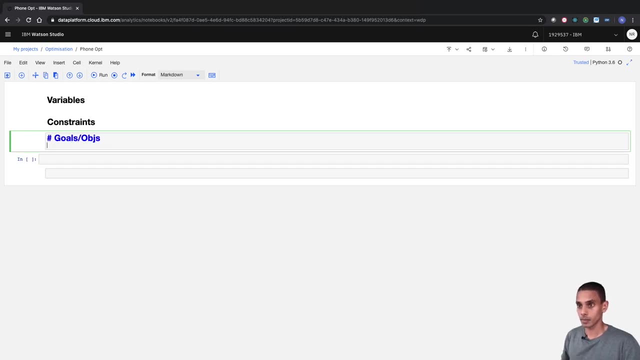 and then we're also going to add in a markdown cell for our constraints, but, not least, we're going to add one for our goals or objectives. Perfect Now, in terms of our variables. we've got a couple of key ones. So, before we actually go and build those variables, 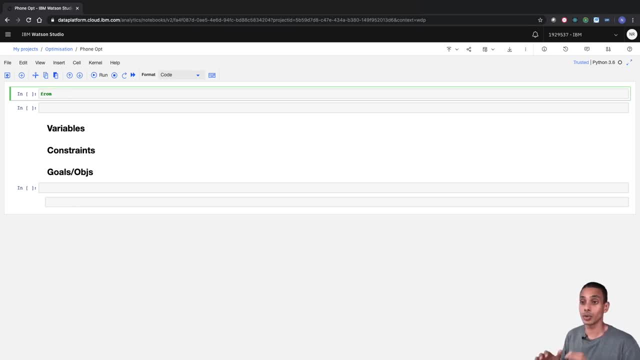 what we want to do is import our dependencies. So to do that we're just going to use the docplex package. So this sort of has a really powerful solver behind it, So that's going to allow us to solve a mathematical problem. So let's import docplex and then from mp and model 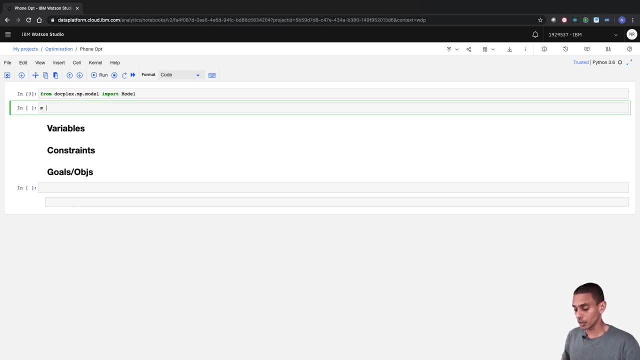 we're going to import the model class. What we're going to do is create an instance of the model, So everything is going to be attached to our model and think of your model as your problem, really. So we'll create a model. 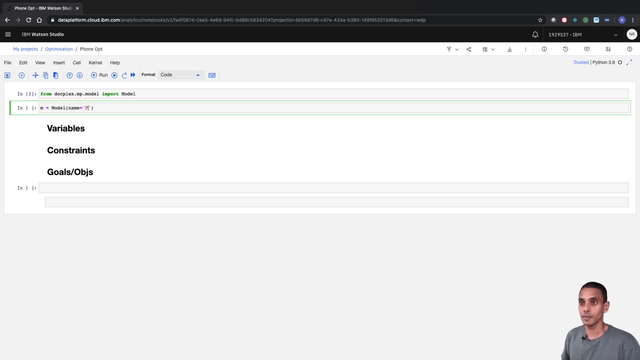 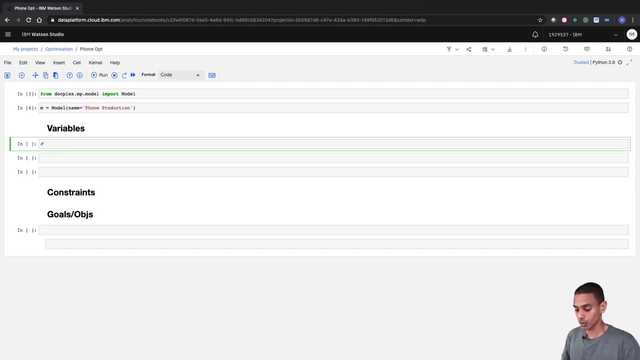 and we're going to name it phone production. and then, within our variables, we're going to name a couple of variables. So, first up, what we're going to do is we're going to create our phone production variables, right? So we have two classes of phones. We had our foldy phone. 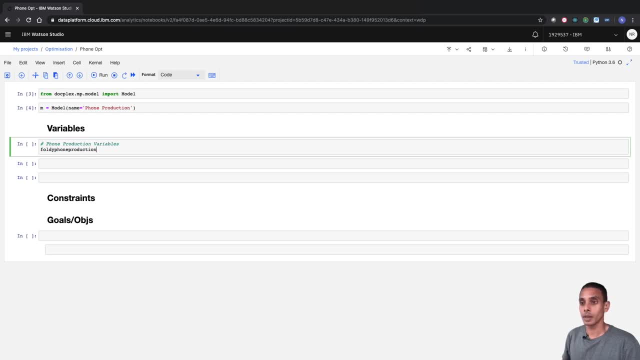 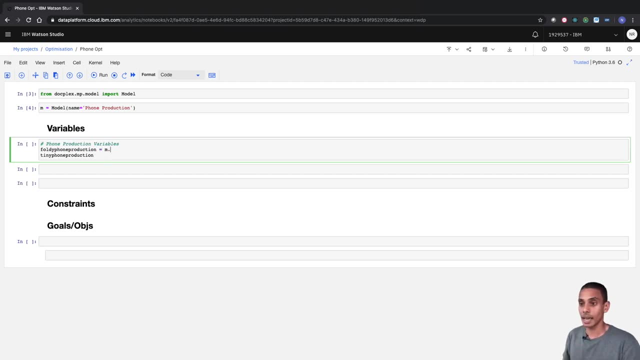 and we had our tiny phone. So let's create two variables for that and add our tiny phone production. Now to create a variable with docplex, all we need to do is type in mcontinuousvariable and we're going to name this as well. So we'll name it foldy. 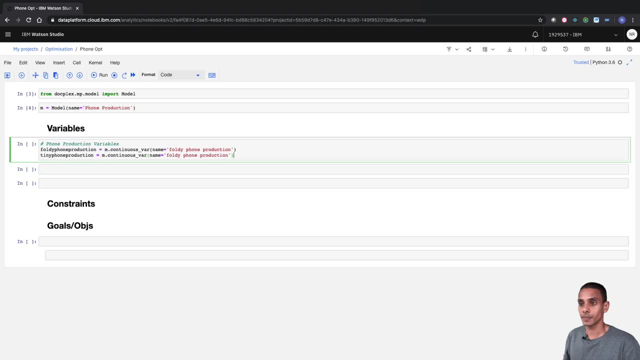 And what we can do is copy that to our tiny phone and rename that tiny phone production- Cool. So we've got our two production variables. Now we had a couple of constants as well that we didn't mention in our problem formulation statement. So what we're going to do is we're 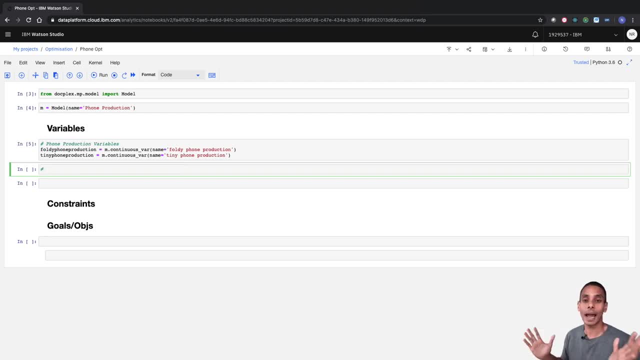 going to do, or our key constraint is really how much time we've got within our manufacturing plant to actually create these phones. So what we want to do is set up a variable that contains how long it actually takes to generate or create one of these phones. So let's create two variables for 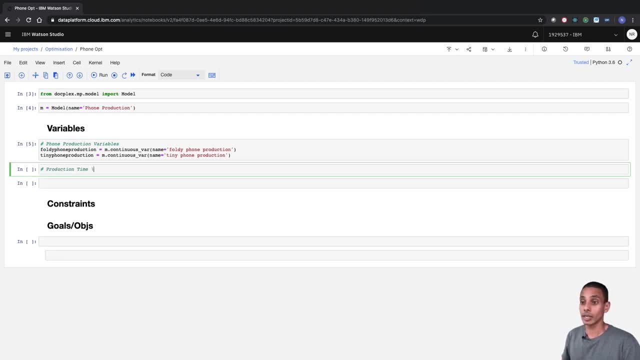 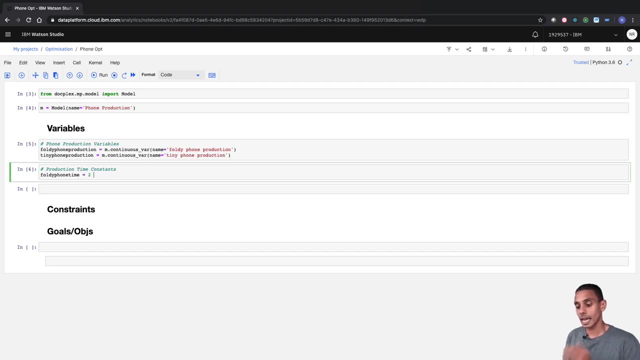 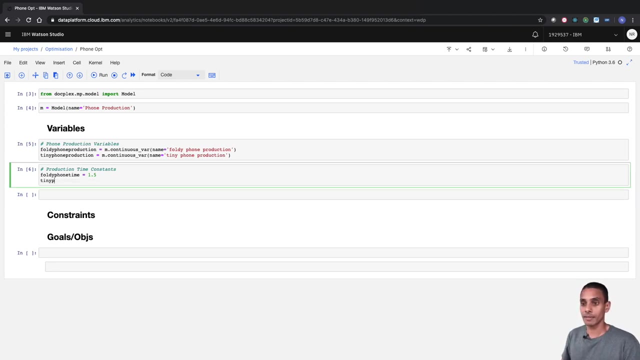 that. So we're going to create- these are actually constants here- and we're going to call one foldy, phone time, and we're going to say that it takes on average one and a half hours to create a foldy. And we're also going to create one for tiny phone And in this case we're going 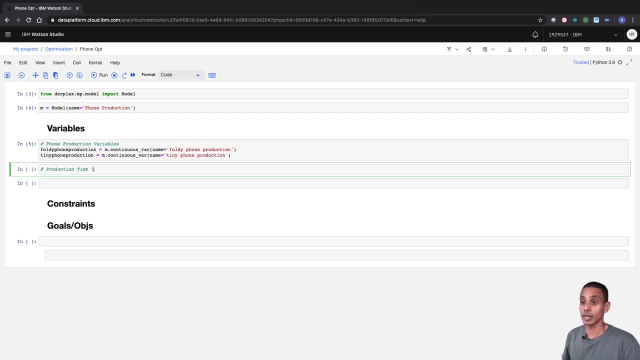 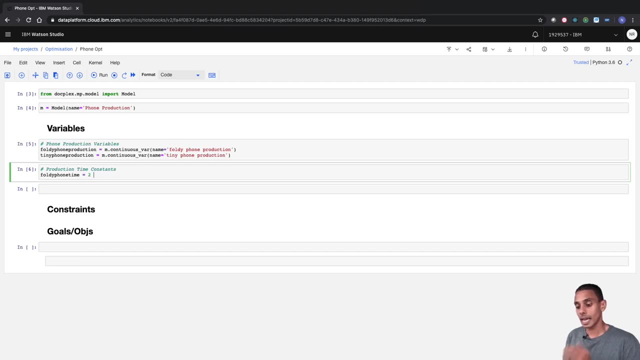 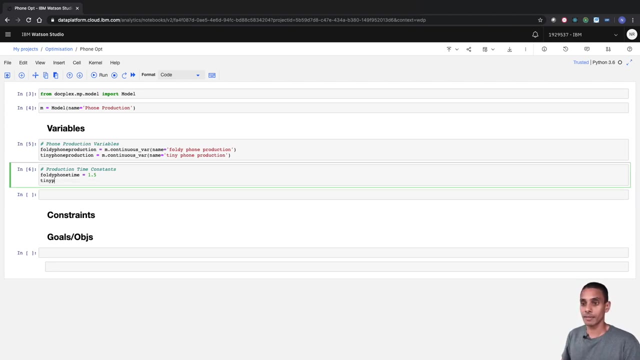 that. So we're going to create- these are actually constants here- and we're going to call one foldy phone time and we're going to say that it takes on average, one and a half hours to create a foldy phone. And we're also going to create one for tiny phone And in this case we're going to say that: 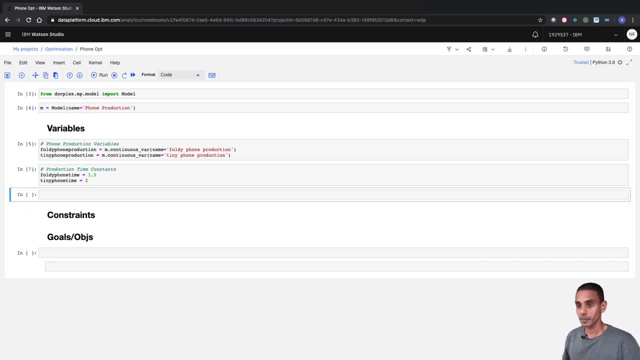 it takes two hours to create our foldy phone or our tiny phone. sorry, Now there's two other constants that we want to add. These are how much sales we're going to generate from each one of these phones. So in this case, we are going to create one for our foldy phone sale price. 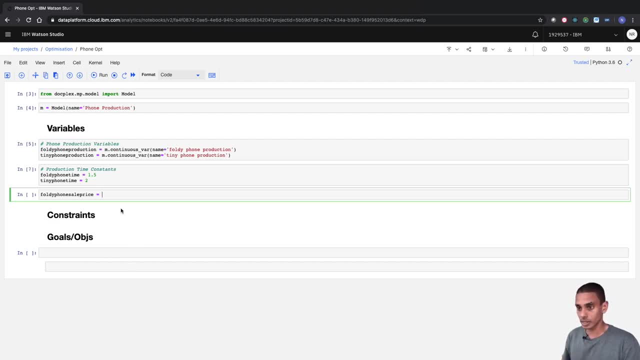 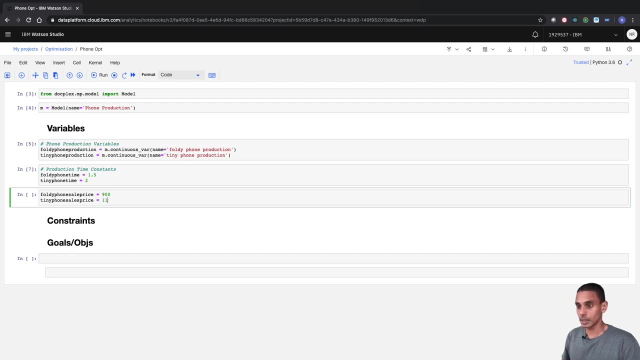 And in this case we're going to say our foldy phone is going to sell for $900.. And we're also going to create one for our tiny phone sales price And we're going to say that one's going to be $100.. 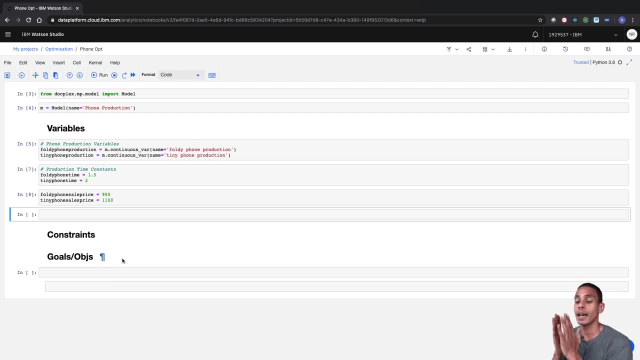 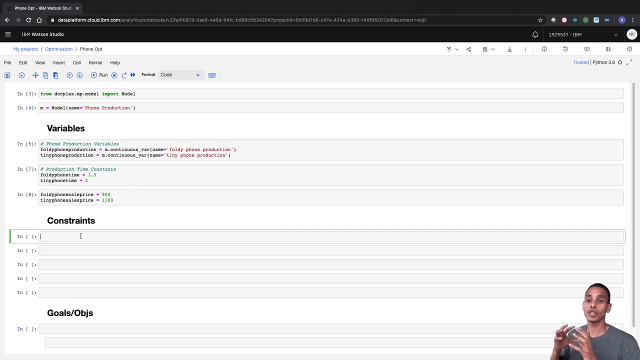 sells for $1,100. perfect, now, that's pretty much all of our variables set up. now what we want to do is start adding our constraints. so at the moment, we know that we need to generate X number of foldy phones and Y number of tiny phones. 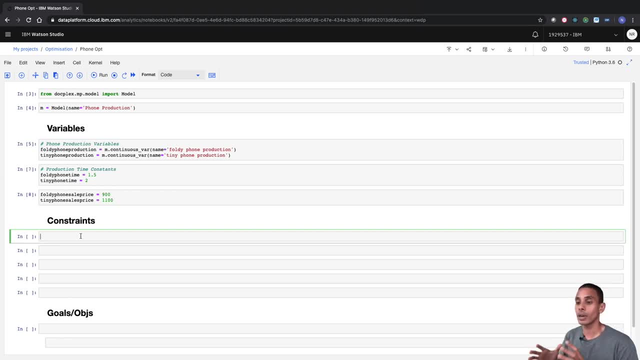 we know that it's going to take one and a half hours to create each foldy phone and about two hours to create each tiny phone, and we also know for every foldy phone that's sold. so, assuming that everything we create is sold, we generate nine hundred bucks, and for every tiny phone that's sold, we generate 1,100. now, 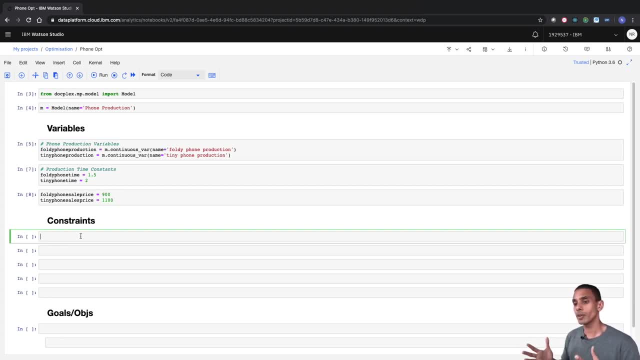 what we're going to do is start to build up our constraints. so remember that we had some contractual constraints. so at a minimum, we need to produce 500 foldy phones, and at a minimum we also need to produce 200 foldy phones. now we also 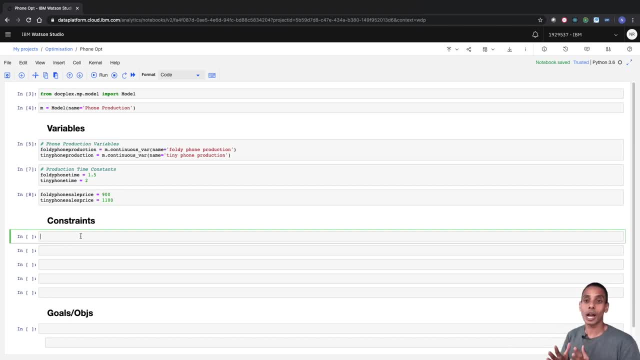 have our production constraints. so we've only got two thousand nine hundred and ninety nine and a half hours to use within our production plan. so let's start modeling up these constraints. so the first constraint that we're going to add is our minimum foldy phone. so we're going to add our minimum foldy phone. 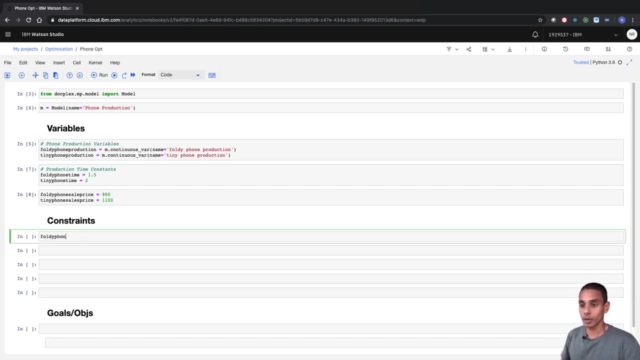 production. so we're going to call that foldy phone constraint, and to do that, we're just going to again append a constraint to our model. now, in this case, what we're going to say is: our foldy phone production needs to be greater than equal to 500, because that's a minimum production level. now we're also 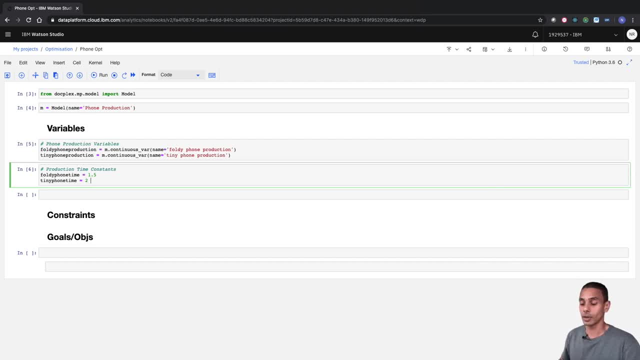 to say that it takes two hours to create out foldy phone or our tiny phone. Sorry. Now there's two other constants that we want to add. These are how much sales we're going to generate from each one of these phones. So in this case, we are going to create one for our 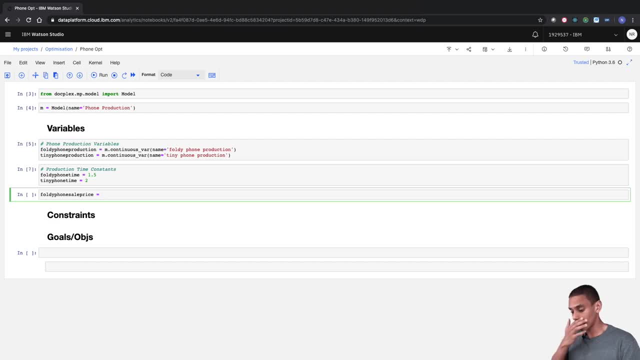 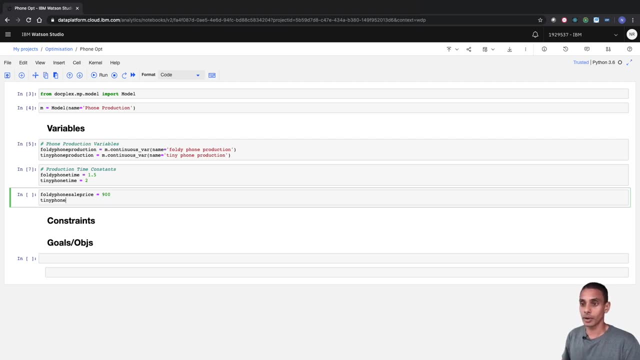 foldy phone sale price. And in this case we're going to say: our foldy phone is going to sell for $900, and we're also going to create one for our tiny phone sales price And we're going to say that one's for. 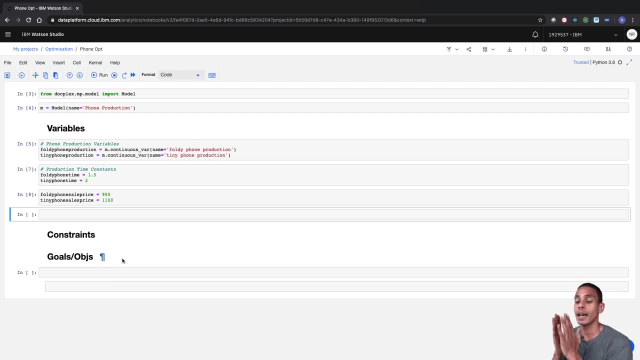 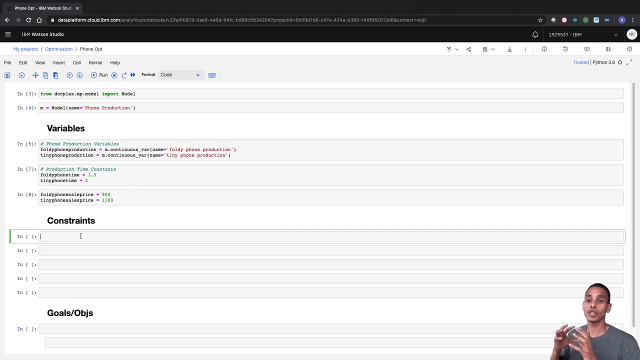 sells for $1,100. perfect, now, that's pretty much all of our variables set up. now what we want to do is start adding our constraints. so at the moment, we know that we need to generate X number of foldy phones and Y number of tiny phones. 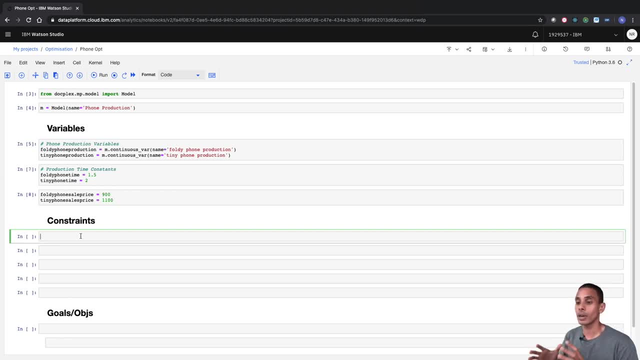 we know that it's going to take one and a half hours to create each foldy phone and about two hours to create each tiny phone, and we also know for every foldy phone that's sold. so, assuming that everything we create is sold, we generate nine hundred bucks, and for every tiny phone that's sold, we generate 1,100. now, 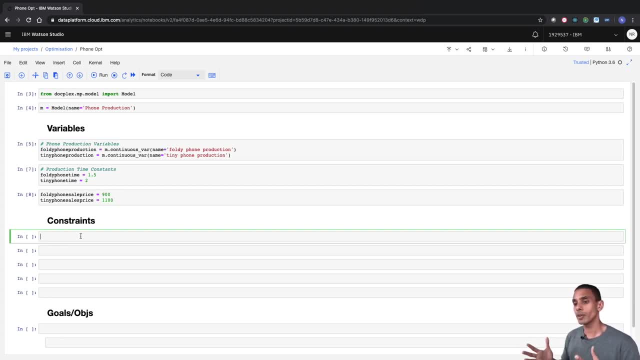 what we're going to do is start to build up our constraints. so remember that we had some contractual constraints. so at a minimum, we need to produce 500 foldy phones, and at a minimum we also need to produce 200 foldy phones. now we also 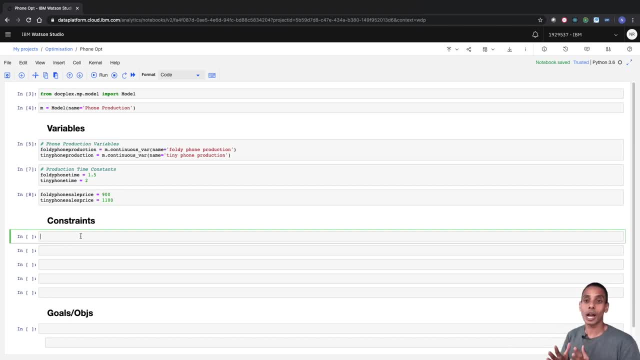 have our production constraints. so we've only got two thousand nine hundred and ninety nine and a half hours to use within our production plan. so let's start modeling up these constraints. so the first constraint that we're going to add is our minimum foldy phone. so we're going to add our minimum foldy phone. 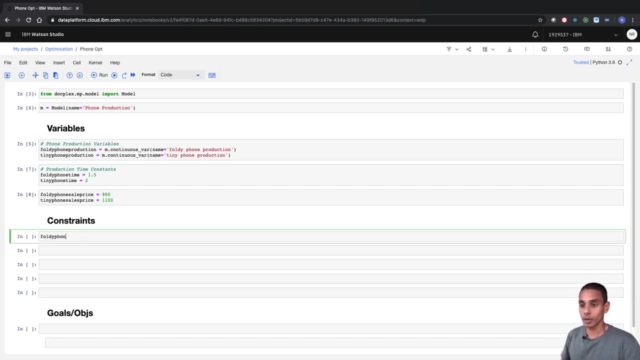 production. so we're going to call that foldy phone constraint, and to do that, we're just going to again append a constraint to our model. now, in this case, what we're going to say is: our foldy phone production needs to be greater than equal to 500, because that's a minimum production level. now we're also 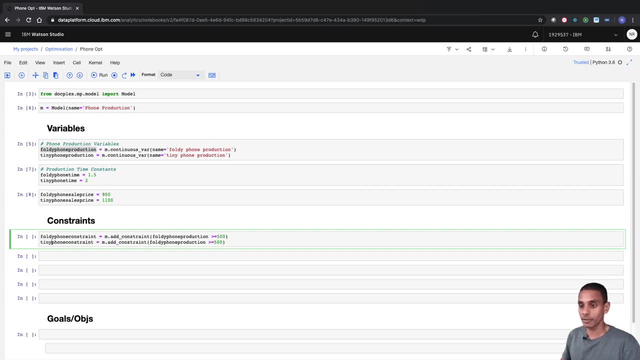 going to add another one, and this one's going to be for our tiny phone production, and in this case we're going to say that our tiny phone production needs to be at minimum 200 phones. perfect, so that's our constraint sort of setup. so we've set up our foldy phone. 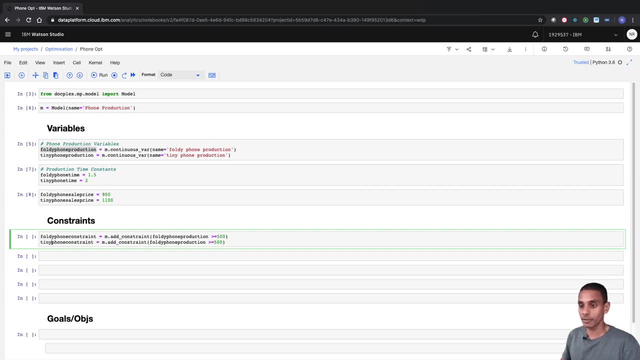 going to add another one, and this one's going to be for our tiny phone production, and in this case we're going to say that our tiny phone production needs to be at minimum 200 phones. perfect, so that's our constraint sort of setup. so we've set up our foldy phone. 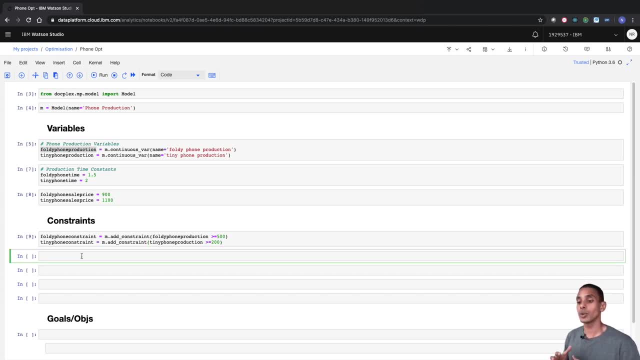 constraint and we've set up our tiny phone constraint. now what we need to do is create a production constraint. so, remember, our production plan has a cap as to how many production hours it's actually got available, and in this case, our cap is two thousand nine hundred and ninety nine and a half hours. so how do? 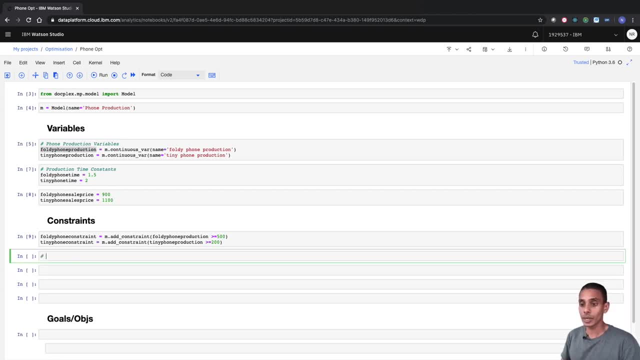 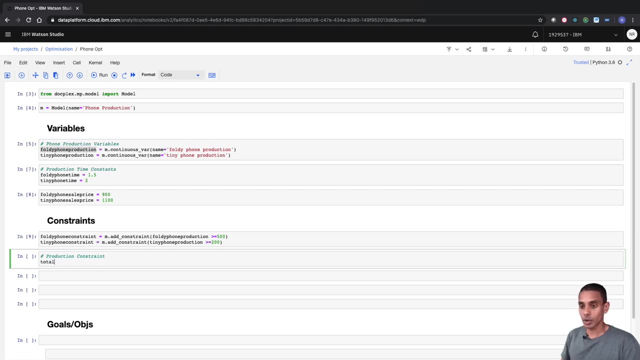 we actually generate this production constraint. well, we can do it in a similar way to how we set up our foldy phone and tiny phone constraint. so what we're going to do is we'll set up a total production constraint and here we're going to add another constraint, and what we're going to say is the sum. 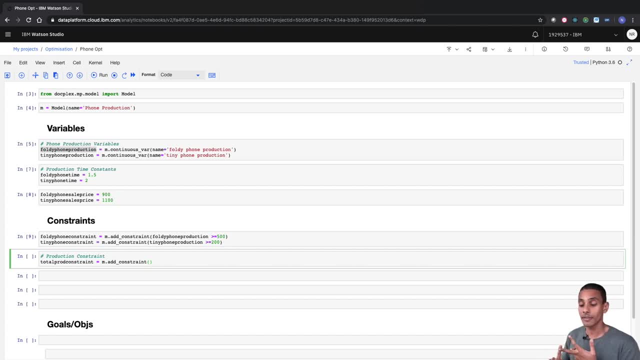 of our foldy phone production hours and our tiny phone production hours must be less than two thousand nine hundred ninety nine and a half hours. so we can do that using the sum formula, and so what we're going to say is the sum of our tiny phone production multiplied by our tiny phone time, plus the sum of our 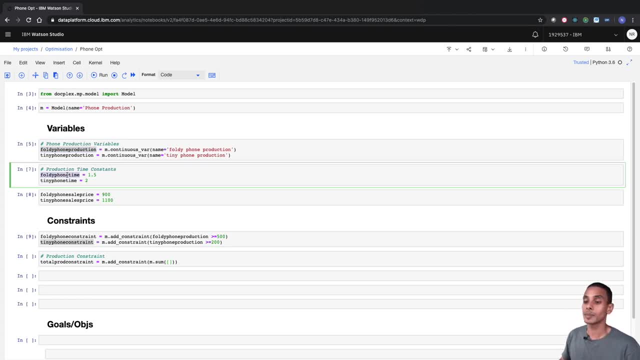 foldy phone production multiplied by our foldy phone time must be less than our production hours. so let's do that. So we're going to say our tiny phone production and our foldy phone production, And so right now we haven't actually added our constraint. 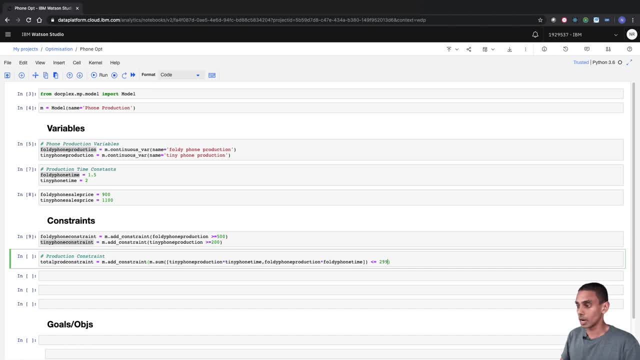 So we're going to say that it needs to be less than 2,999 hours, 299 and a half hours, And that's basically our last constraint done. So now, what we've done is we've set up our foldy phone constraint. 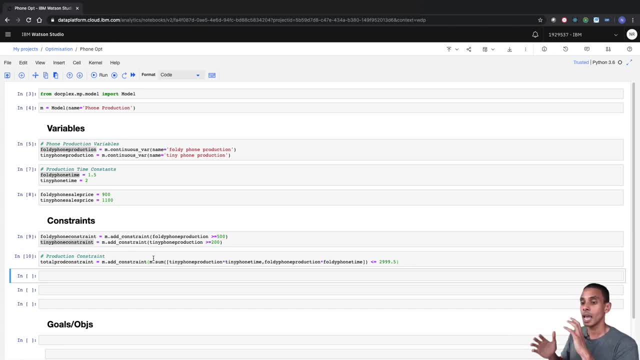 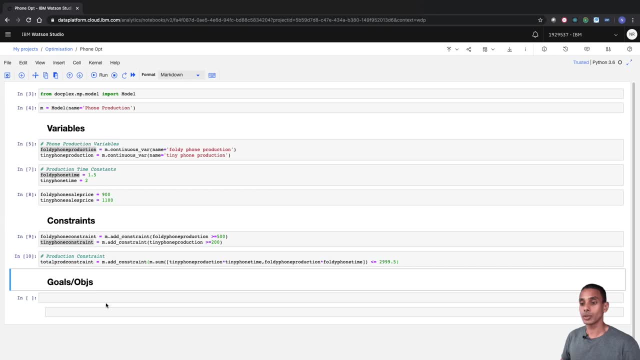 So we're going to meet our minimums, our tiny phone constraint- again our minimums- And we've also set up our overall production constraint. So that's really our constraints sort of set up. Now the last thing that we need to do is specify our goal or objective and then solve our problem. 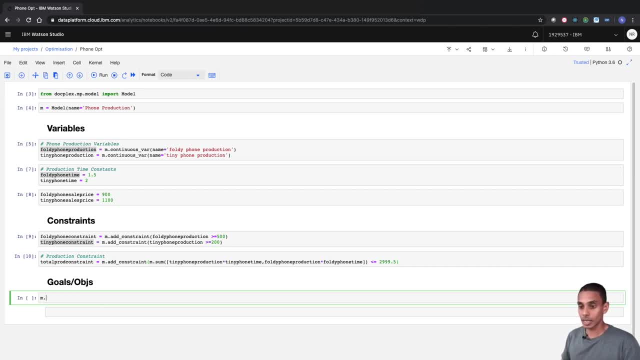 So in this case we're trying to maximize the value of sales. So what we're going to do is maximize our sales formula. So in this case, our sales formula is really our foldy phone production multiplied by our foldy phone sales price. 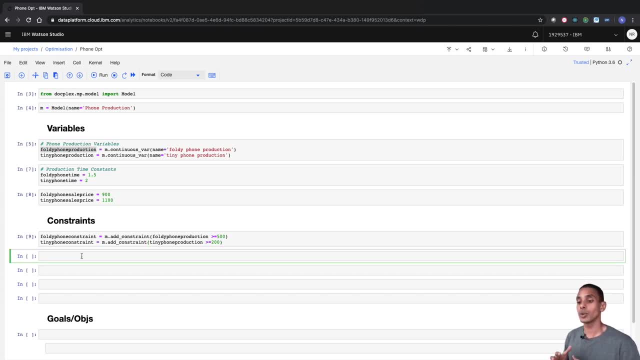 constraint and we've set up our tiny phone constraint. now what we need to do is create a production constraint. so, remember, our production plan has a cap as to how many production hours it's actually got available, and in this case, our cap is two thousand nine hundred and ninety nine and a half hours. so how do? 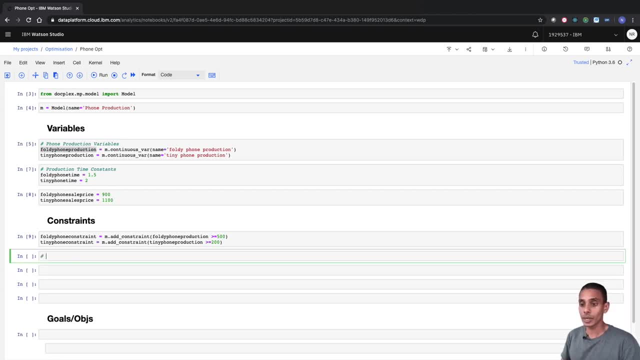 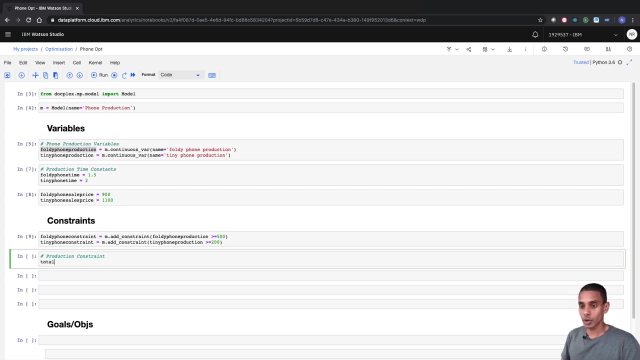 we actually generate this production constraint. well, we can do it in a similar way to how we set up our foldy phone and tiny phone constraint. so what we're going to do is we'll set up a total production constraint and here we're going to add another constraint, and what we're going to say is the sum. 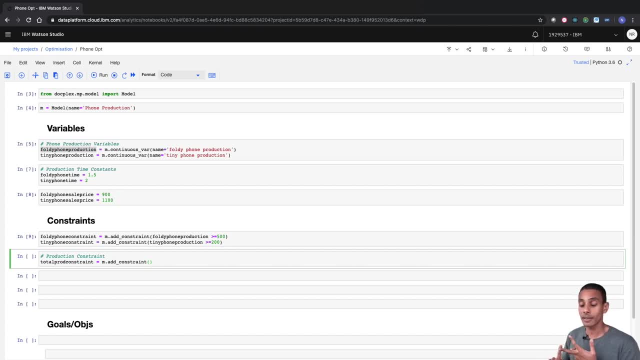 of our foldy phone production hours and our tiny phone production hours must be less than two thousand nine hundred ninety nine and a half hours. so we can do that using the sum formula, and so what we're going to say is the sum of our tiny phone production multiplied by our tiny phone time, plus the sum of our 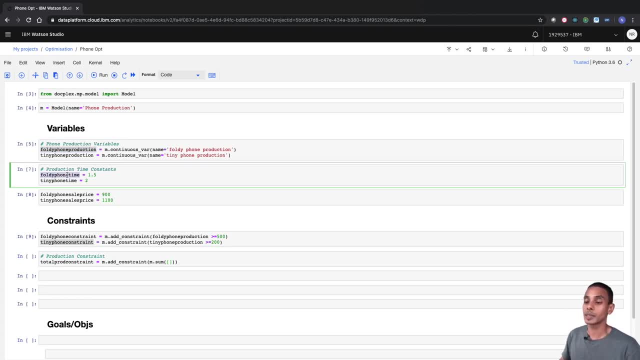 foldy phone production multiplied by our foldy phone time must be less than our production hours. so let's do that. we're going to say our tiny phone production and our foldy phone production, and so right now we haven't actually added our constraint, so we're going to. 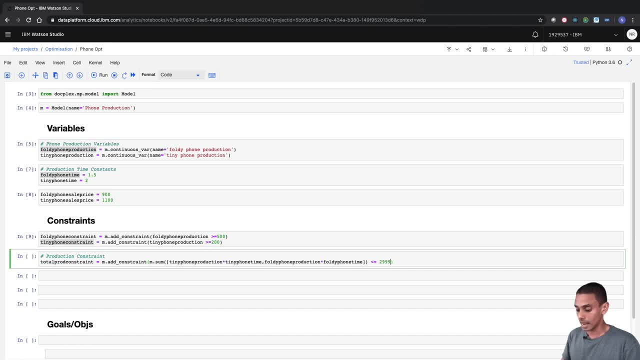 say that it needs to be less than two thousand nine hundred and ninety nine hours, two hundred ninety nine and a half hours, and that's basically our last constraint done so. now what we've done is we've set up our foldy phone constraint, so we're going to meet our minimums, our tiny phone constraint, again. 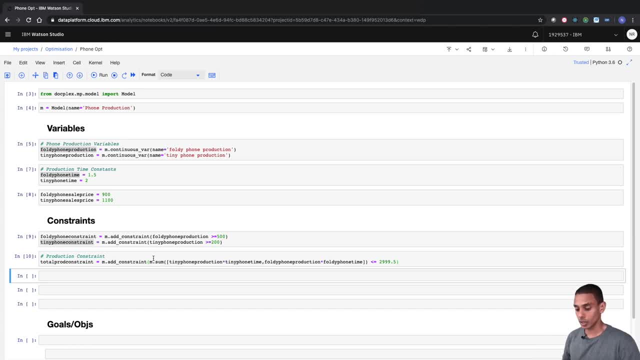 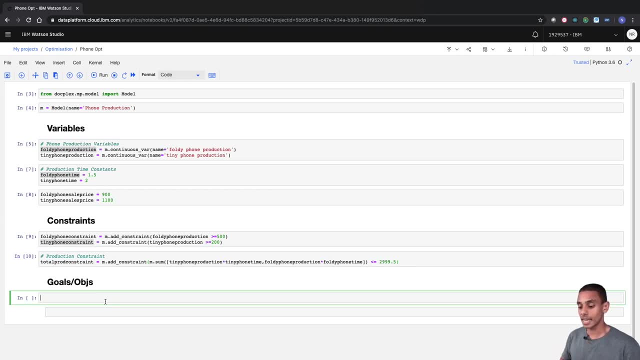 our minimums and we've also set up our overall production constraint. So that's really our constraints sort of set up. Now the last thing that we need to do is specify our goal or objective and then solve our problem. So in this case, we're trying to maximize the value of sales. So what we're going to do is 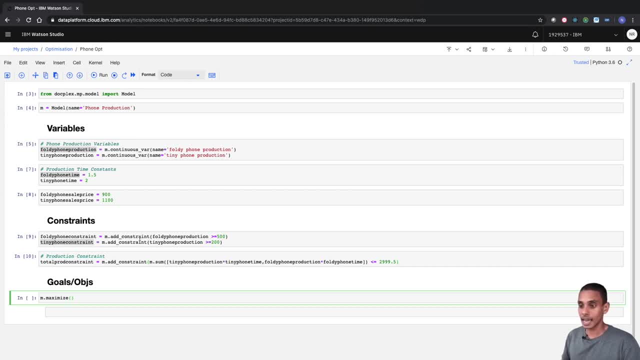 maximize our sales formula. So in this case our sales formula is really our foldy phone production multiplied by our foldy phone sales price, our tiny phone production multiplied by our tiny phone sales price. So this sort of assumes that we sell all of the phones that we actually